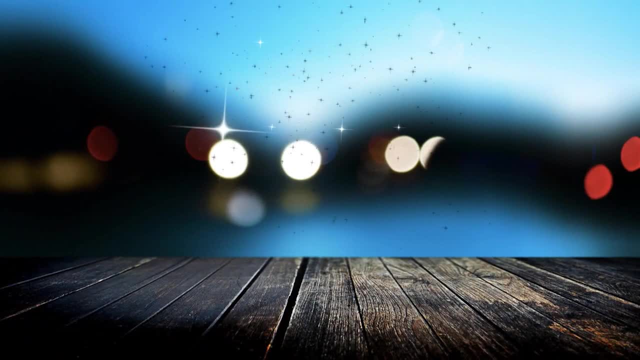 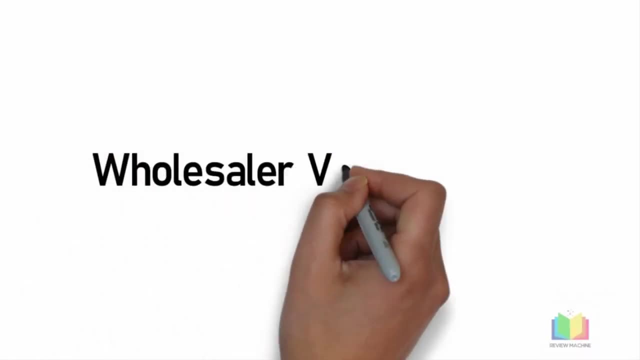 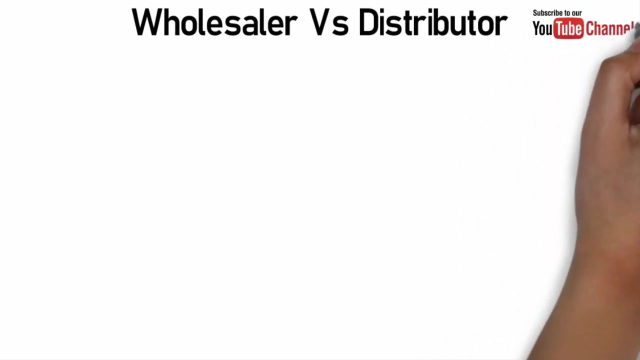 Hi friends, welcome to my channel, and in today's video let us discuss about the difference between a wholesaler and a distributor. So before beginning the video, I request you to please subscribe to my channel so that you will get notified whenever I upload a new video. So here: 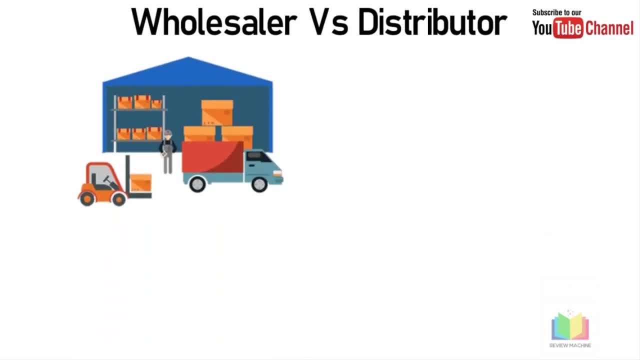 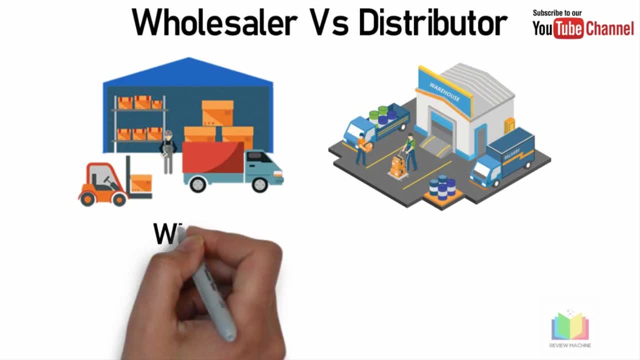 in this video we will define the term wholesaler and a distributor, and then we will understand the key difference between a wholesaler and a distributor. So first let us understand the term wholesaler. So a wholesaler is a trader who buys the goods in bulk quantities and then he 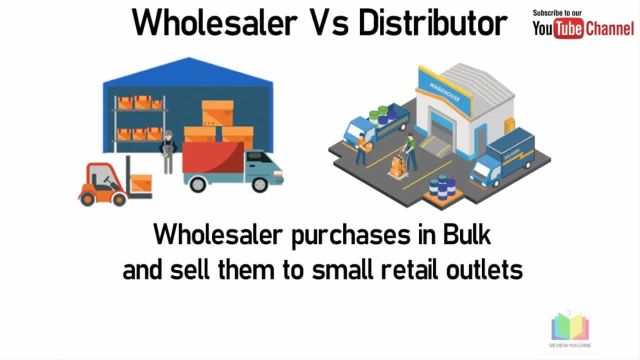 sells them in a relatively smaller units. The customers for the wholesalers are mainly small retail outlets and kirana shops. Also, the serving area for wholesalers is limited in comparison with the distributor, Whereas a distributor is someone who is engaged in supplying goods and services to various businesses and customers. So the distributor is someone who is engaged in supplying. 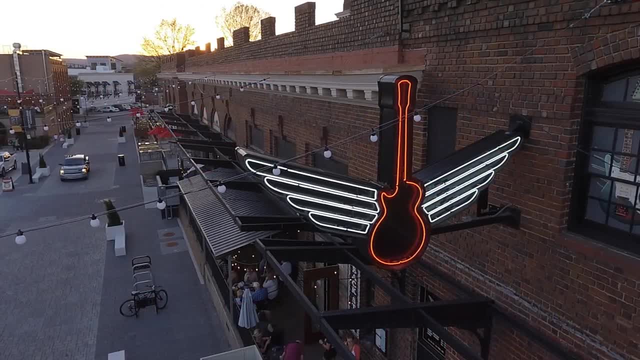 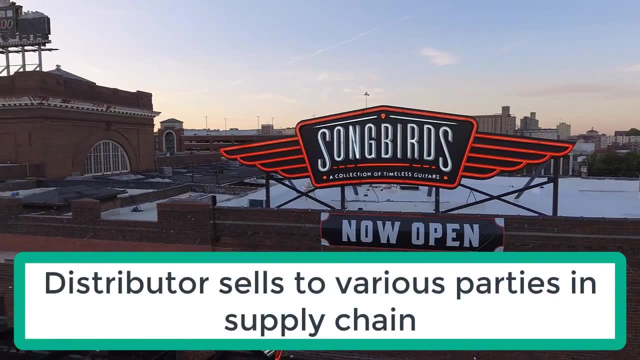 goods and services to the entire market, But for a wholesaler the area is very specific where he is going to sell the merchandise. The distributor is an agent who distributes the products and services to various parties in the supply chain network. We have to understand that it is impossible. 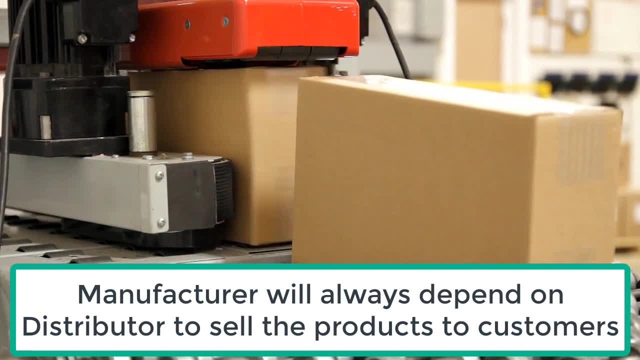 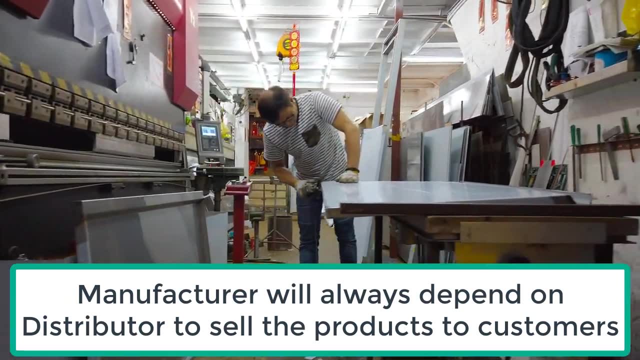 for a manufacturer to reach customers directly for selling of the products. So, because of this, they have to depend on the distributors, who will further sell it in different locations. So, friends, this was the definition of wholesaler and a distributor. Now let us see the definition of wholesaler and a. 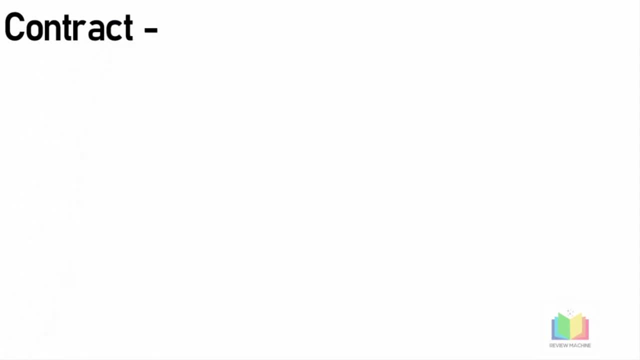 distributor. So now let us understand the difference between these two terms. So the first key difference is with respect to the contract, That is, the distributor will enter into the contract with the manufacturer to trade in for the product lines, But whereas a wholesaler will not enter into any. 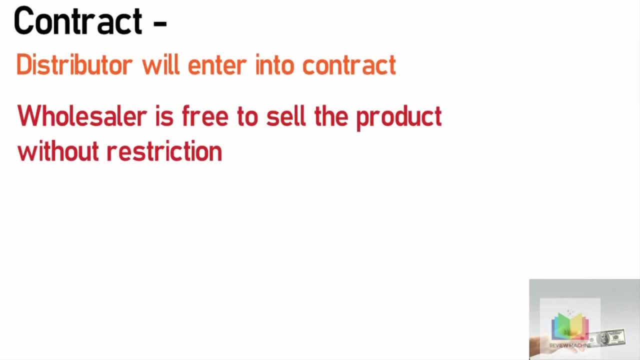 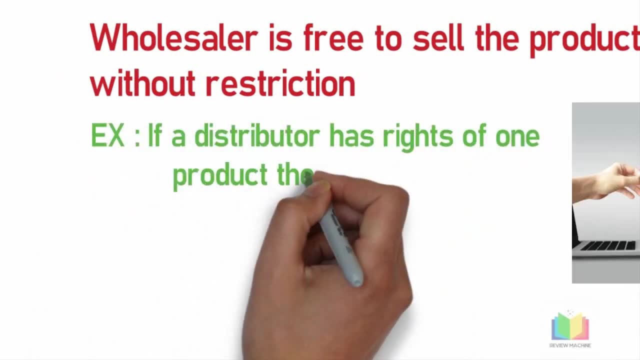 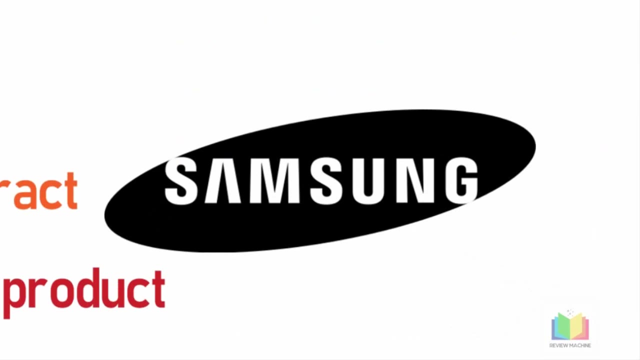 contract with the manufacturers. That is, a wholesaler can sell products provided by various manufacturers and distributors. For example, if an electronic distributor has taken distribution rights of samsung products, then he can sell only samsung products in the market, But whereas a wholesaler can sell products of various brands, That is, the wholesaler is not restricted to one. 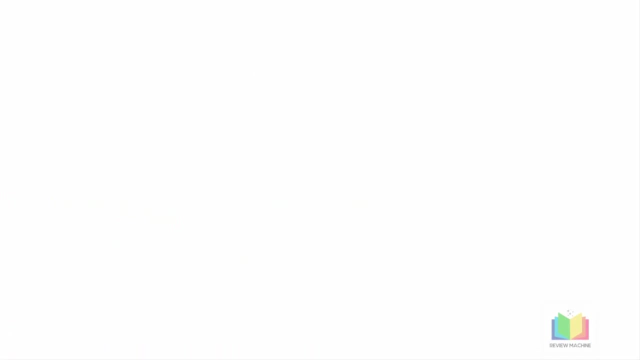 particular brand or one particular company. So the next key difference is with respect to the customers. That is, the wholesaler will have only retailers as their customers and, on the contrary, distributor provides goods to many parties in the supply chain, Like he will supply goods to wholesalers.